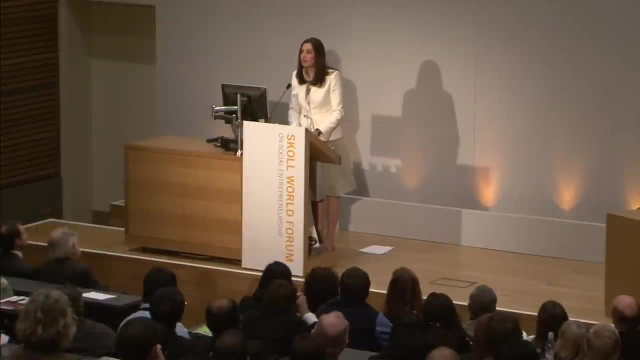 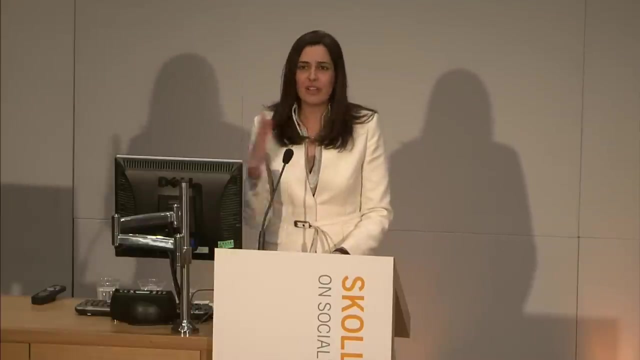 text descending from heaven to mankind on earth was read- Read in its many senses, to learn to observe and, most important, to eradicate ignorance from mankind's mind. and how far we have drifted from that first moment where education and learning was so critical and where we are. 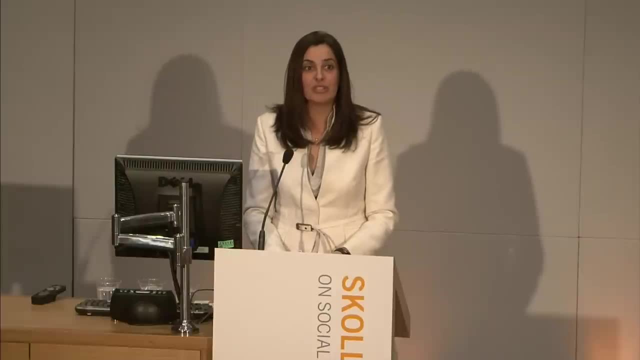 today, the education systems across the Arab world have failed. It's youth: 200 million. We are a population of 300 million. 70% are youth. and what it looks like from the video that you showed us that we exported the golden age of Islam and imported 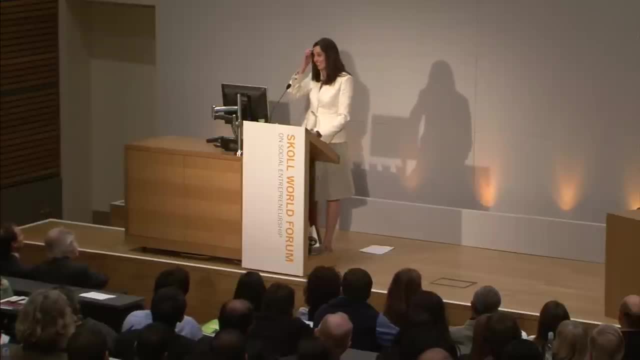 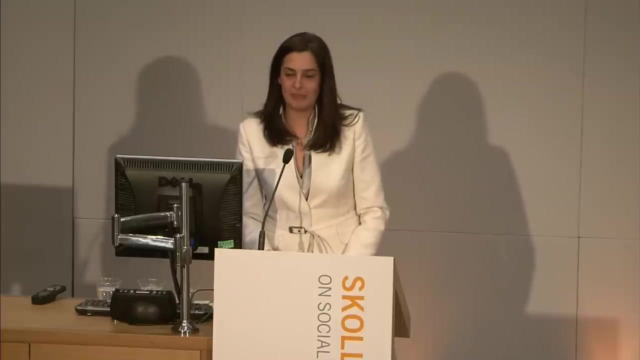 an archaic education system from the industrial revolution. So I don't know. You thank me, and I. So the golden age of Islam was a truly, and I mean we must go back to it to understand what was happening with. It was a period where people from different religions, from different cultures were coming. 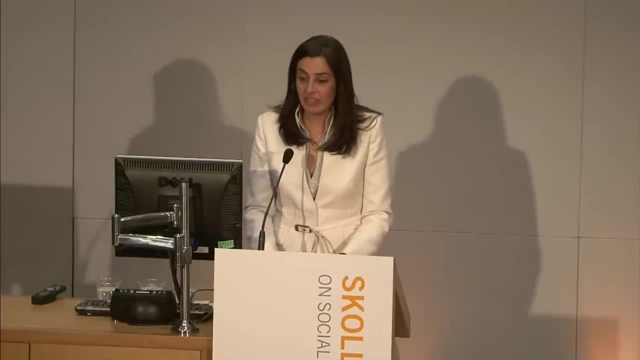 together to move humanity forward. and today we have an education system that is forcing memorization, that's government see that education is the sole responsibility of government and that the youth Are there Just to memorize, take exams and, as you mentioned, completely isolated from the ability to. 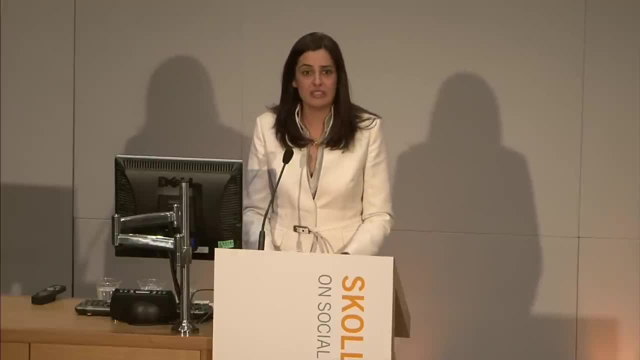 even think about the issues that surround their communities and surround their countries, from water issues in our region to even employment issues, and what this has created is the worst unemployment issue amongst youth in the world. The Arab world has between 30 to 40 percent unemployment amongst its use, Even And when we had the oil boom of 2007 and early 2008 and Employment in Saudi Arabia, amongst the US, with 30 percent. in the United Arab Emirates, where every expatriate was going there to make their money, 32 percent unemployment amongst its use and, in nine, all producing 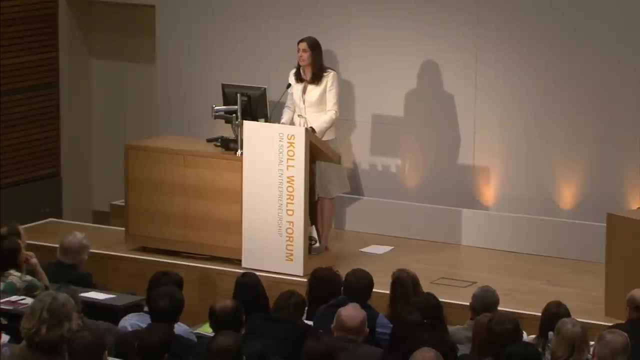 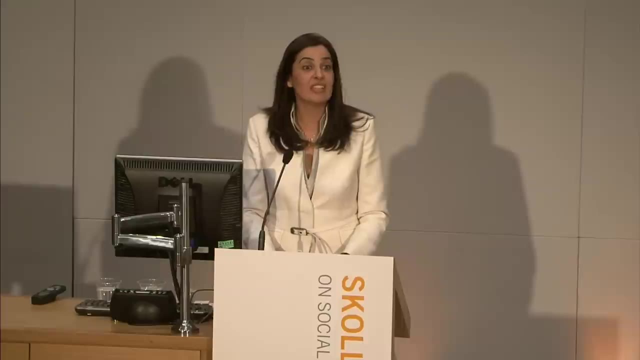 countries: Algeria, 40 percent, Syria, 37 percent, even in Jordan, and 30 percent unemployment. amongst its use, We have become experts in the marginalize of youth and the irony of it is just recently, just this last week. I reports from seven. six hundred CEOs surveyed across the region, their number one. 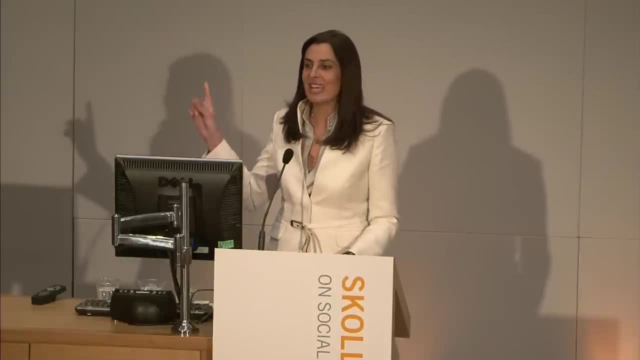 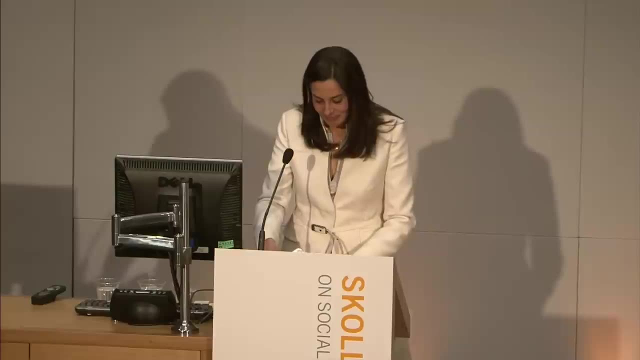 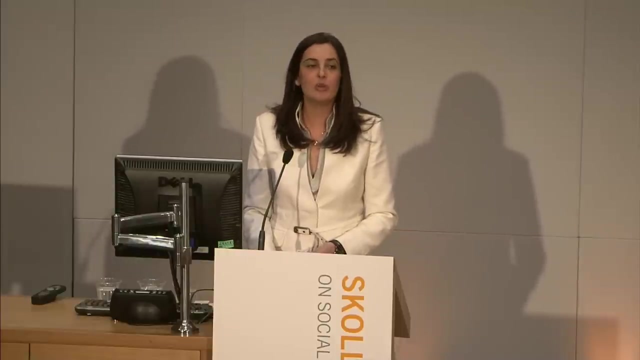 obstacle to growth: qualified human capital. what do we do? Brookings Institute, in 2003, puts a report out called the youth factor, and what they said is those that will control and politically mobilize the youth of the Arab world will be the ones that will win in the end. is it going to be a? 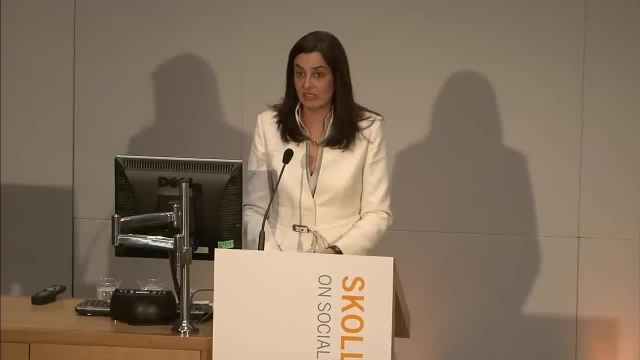 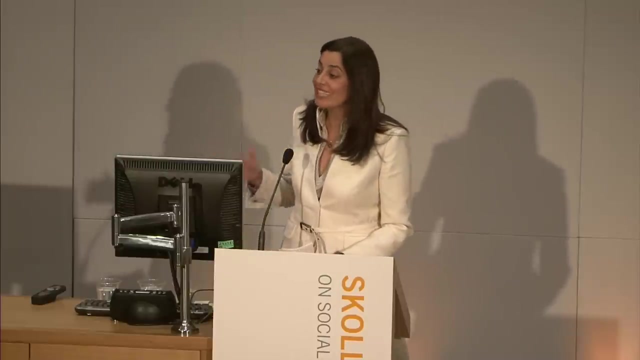 government, or is it going to be the Islamists? and the World Bank said over the next, until the year 2020, 80 million new jobs must be created, when the current labor market is 54 million jobs that needed 50 years to create and in less than 15 years we have to create 80 million jobs. what Brookings? 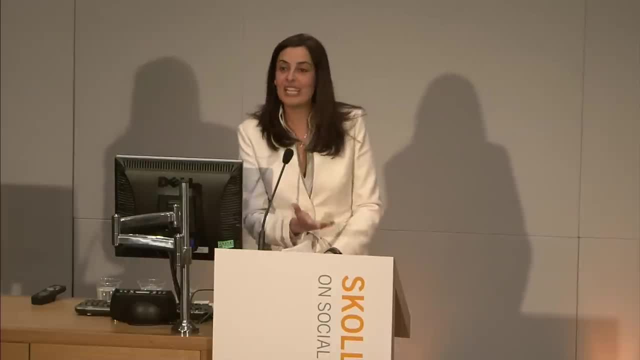 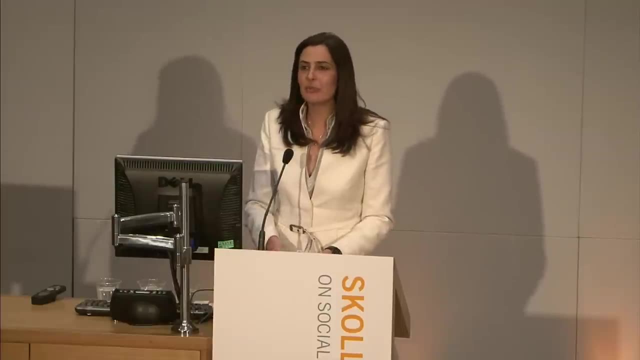 did not realize in 2003, but a silent movement was mobilizing from Jordan, as Pamela mentioned, where Queen Rania helped us from inception and realized the importance of investing in youth. she volunteered in our classrooms and drove the private sector to follow. she invited them to vote to to follow, and a hundred and seventy corporations just in. 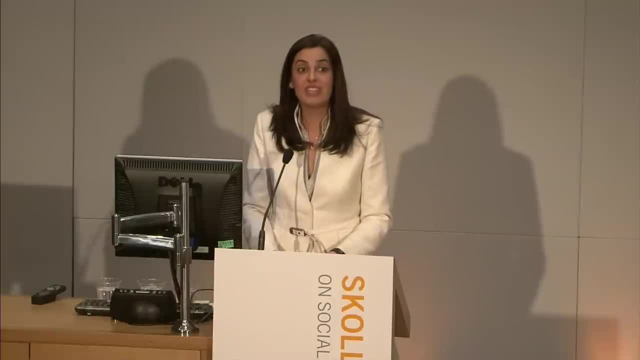 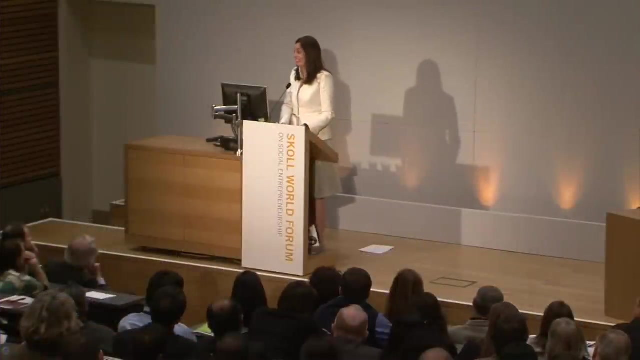 Jordan followed suit, mobilizing more than 3,000 volunteers into the classroom, and today Jordan reaches 36% of high school. students are now being taught skills of the 21st century. it's about time, isn't it? entrepreneurial skills, financial literacy, workforce readiness and with. 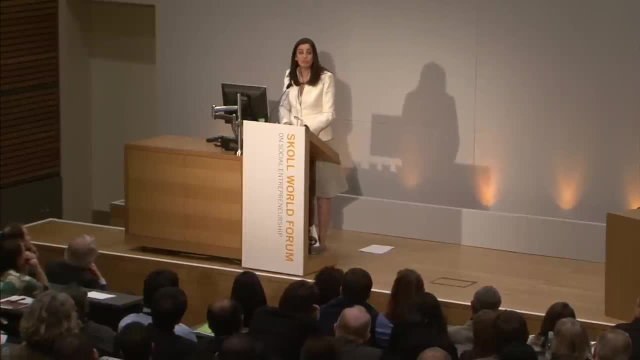 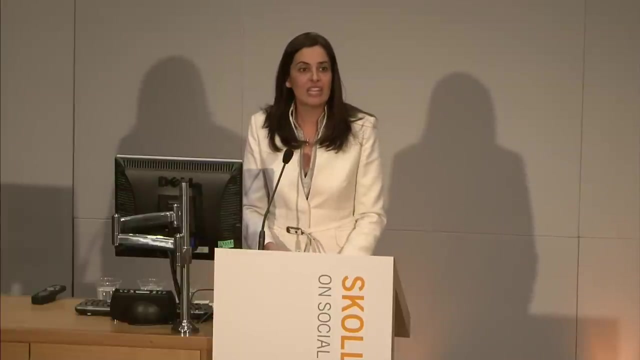 complete passion and dedication. it has become a movement. every person who has made it owes it to the next generation to go back in there and lift them with the skills that they have and what we found- this from Jordan since 2005 until today. in the last four years we have mobilized like fatty can do it, I'm sure. 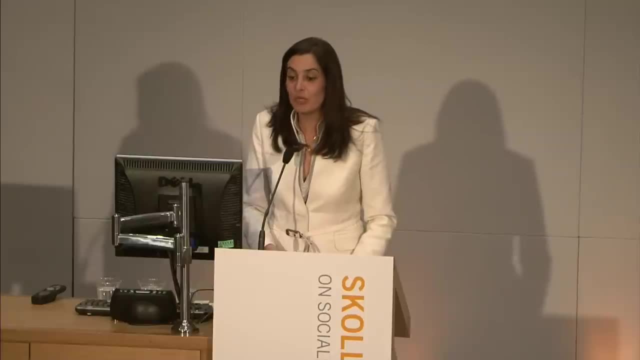 you're here and his Rolodex that these days is more important than any other days is more important than an oil well, and we mobilized its contact list to move across the region, meeting business leaders from across 12 Arab countries and, today, 12 ministries of education, some of which took three and a half. 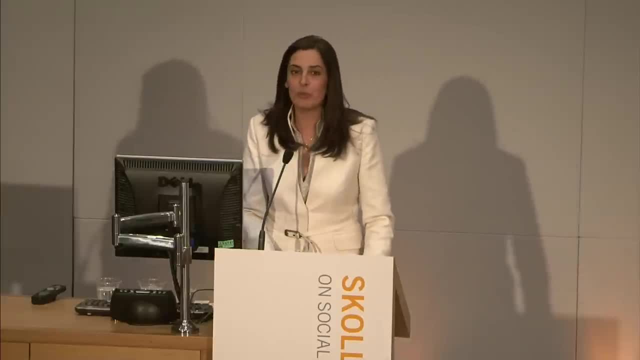 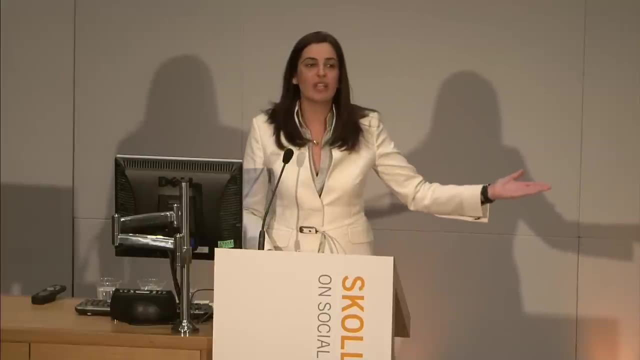 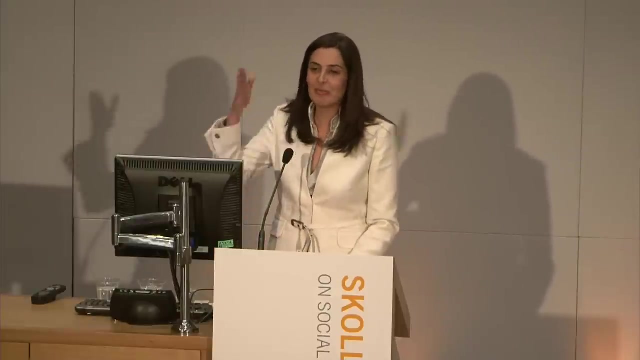 years to open the door and we kept at it, from one business leader to the next helping us. today, 12 ministries of education have opened their doors wide open to the Arab private sector to say welcome. we finally acknowledge that it's time to partner with you and for your staff that you have invested in to go. 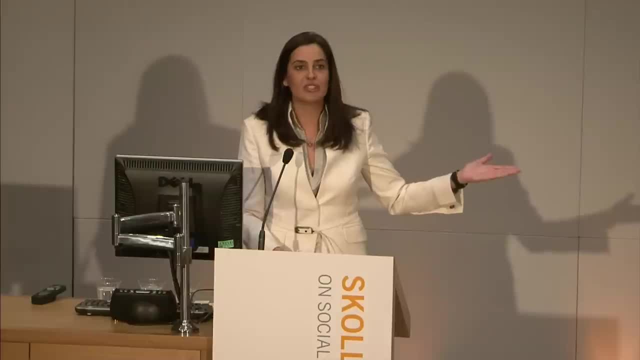 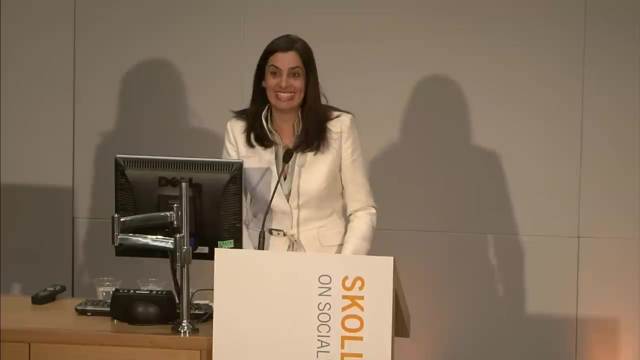 into the classroom to teach the youth of their world how to succeed in the private sector. I want to take this opportunity to thank Her Majesty Queen Rania for finally creating a coalition of the powerful, and this time not for war but for peace and for the next generation of the Arab world. last year, at the world economic 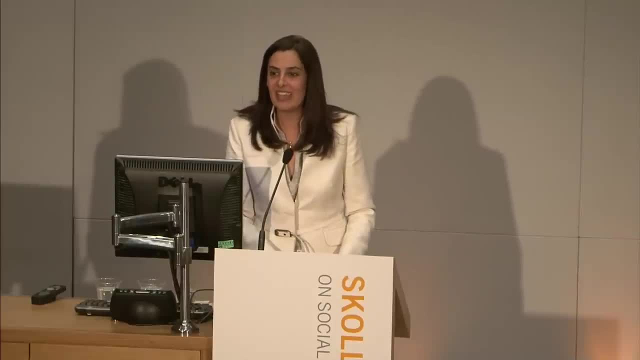 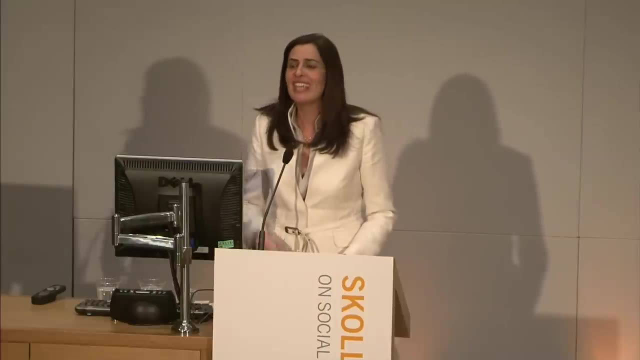 forum in Davos, we invited the top leaders of multinational corporations and Arab business leaders to come together. if you are doing business in the Arab world, invest in the Arab world. just send your staff into a nearby school, and with that we launched our road to reach 1 million Arab youth each year, to create a 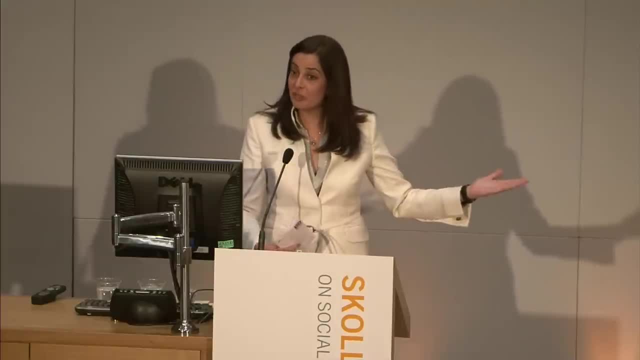 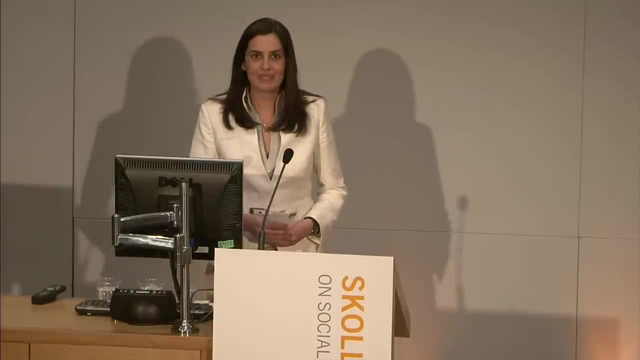 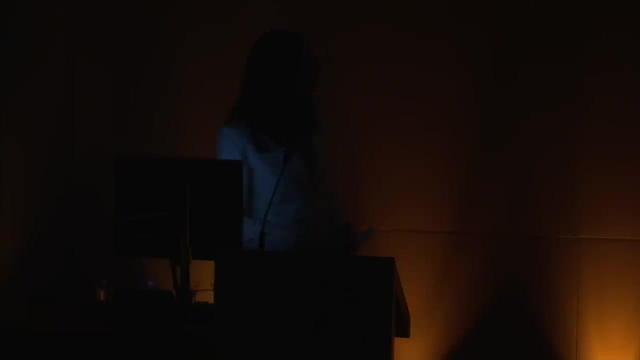 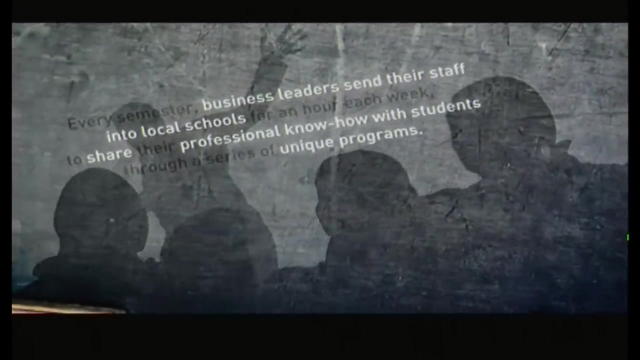 new face to the Arab world and I would like to preview the new face of the Arab world. there's a documentary from every semester. business leaders and their staff to local schools for an hour each week to show their professional hands with students through a series of unique programs, by starting up and operating an actual 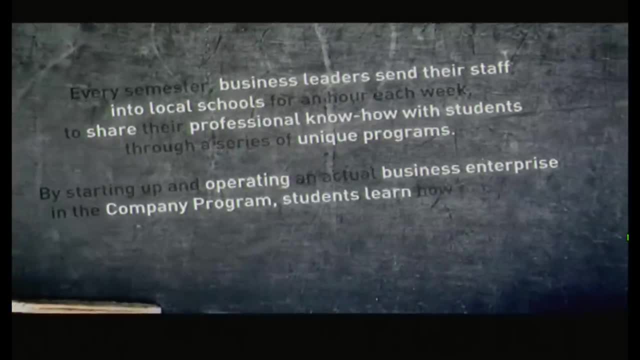 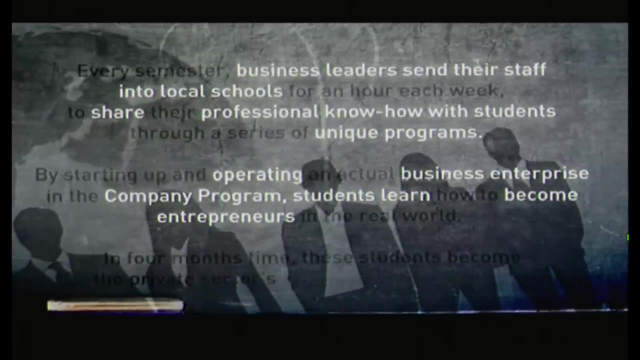 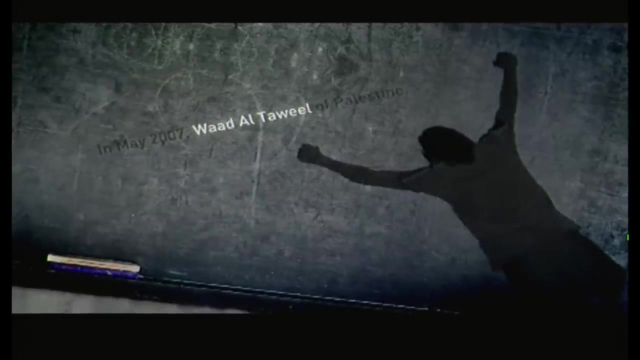 business enterprise and a company program, students are now to become entrepreneurs in the real world. months time, these students become the private sector's most valuable investment. in may 2007 of palestine led her classmates to victory after a three-day intense grilling by a jury of arab ceos. 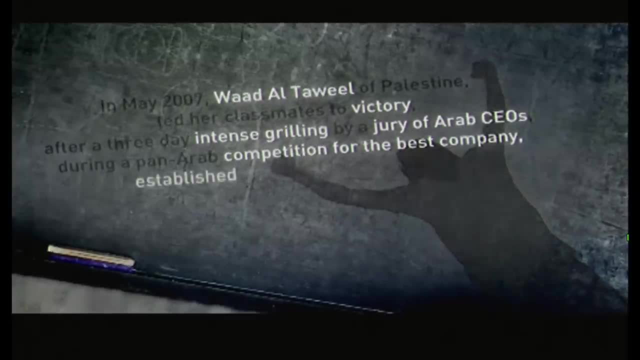 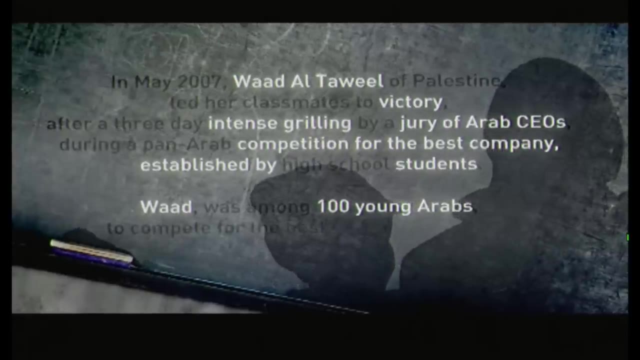 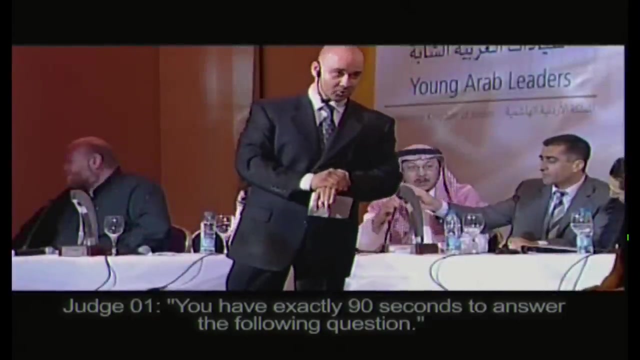 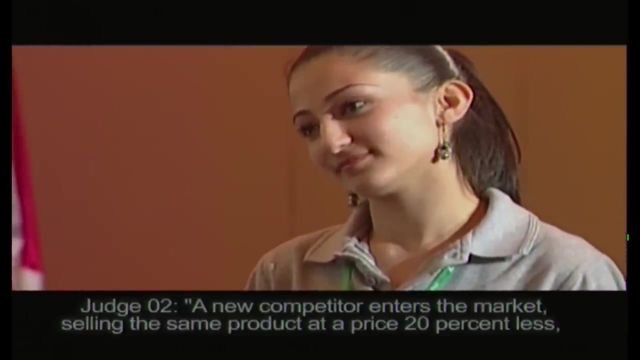 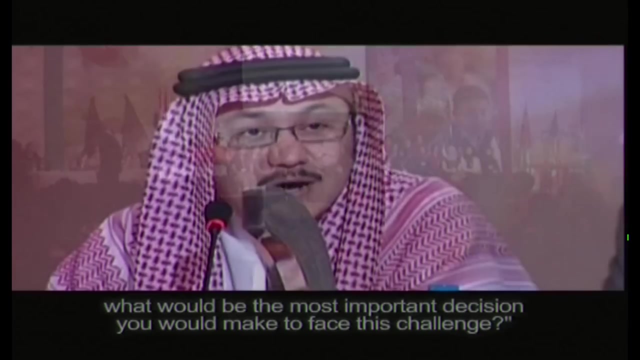 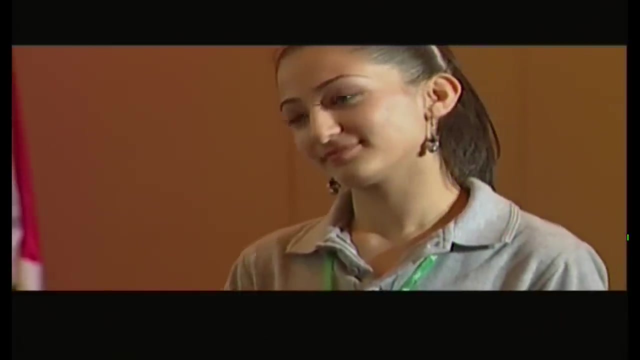 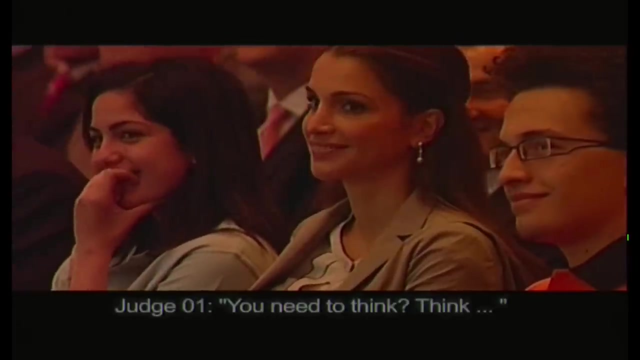 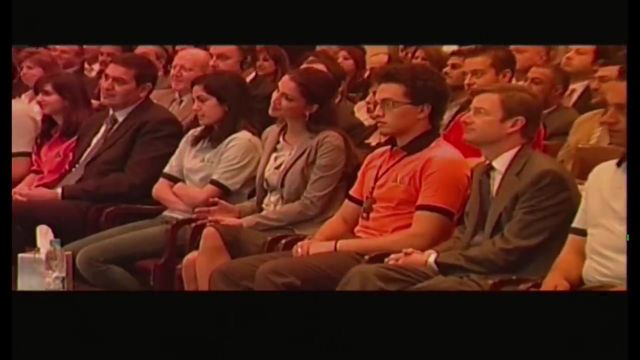 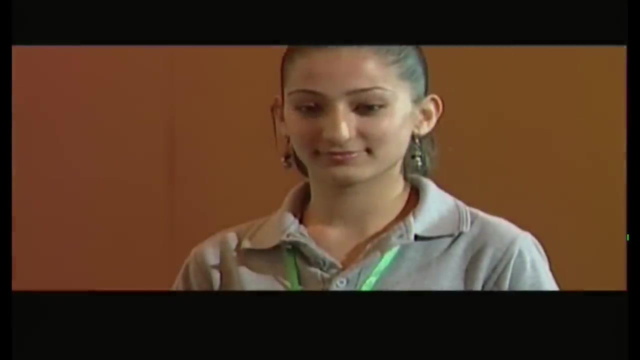 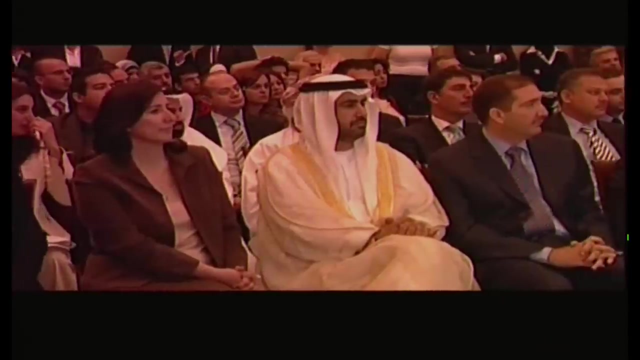 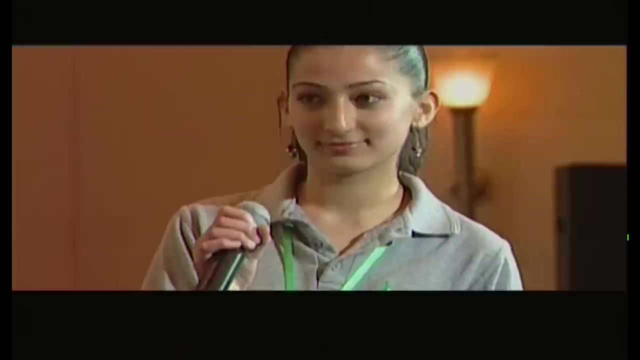 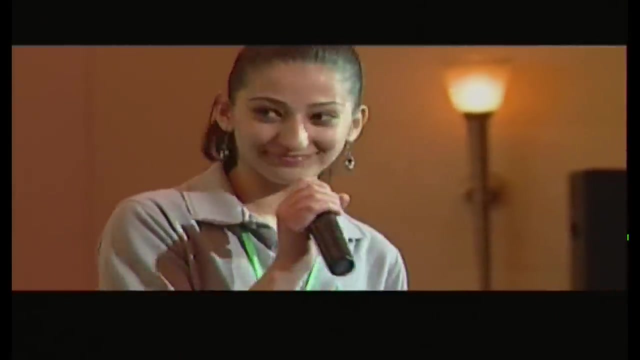 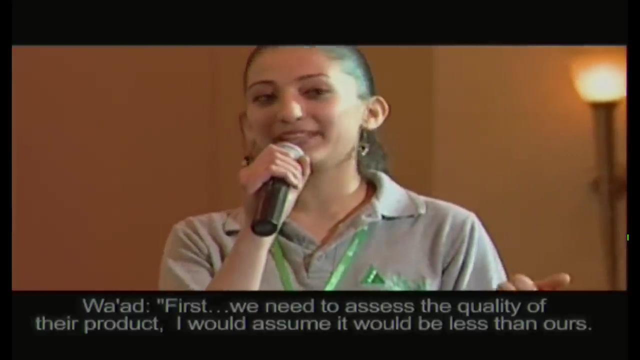 during a pan-arab competition for the best company established by high school students, waad was among 100 young arabs to compete for the best student ceo title. a ham karar sofa. ttk dina be hadil hala uh. If they came to us with a product that was cheaper than ours, we should first see the quality of their product. 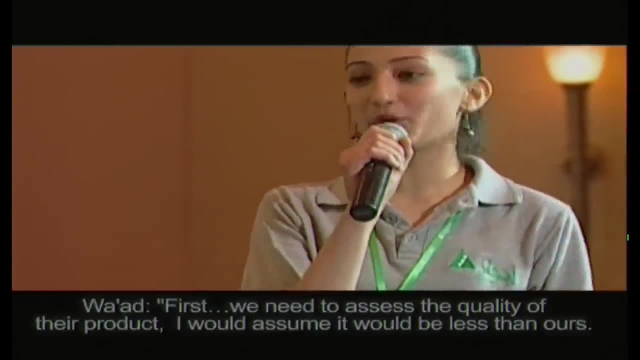 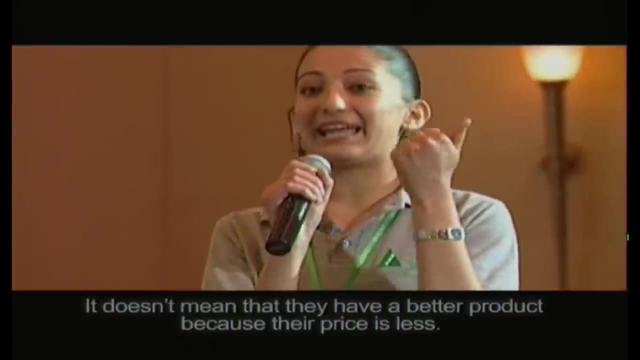 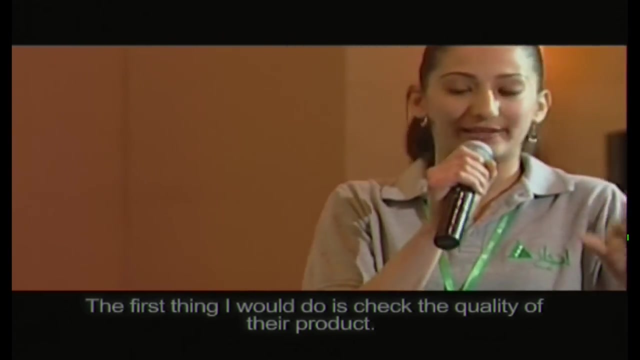 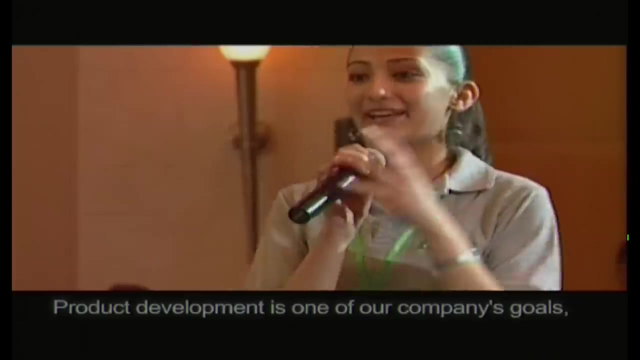 If the quality of the product is better than ours, we can change the quality of the product and improve it, Or we can make some adjustments to the price of the product to match the current market price. We should do these two things. Product development is one of the goals of our company. 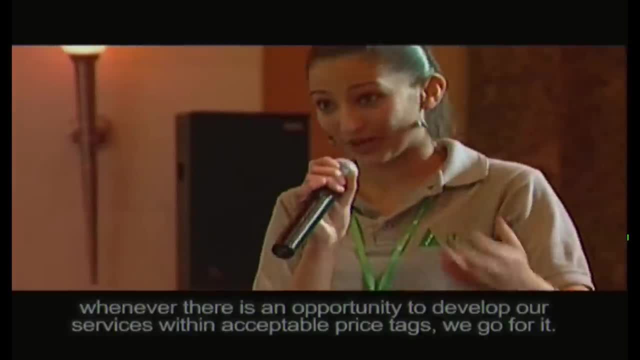 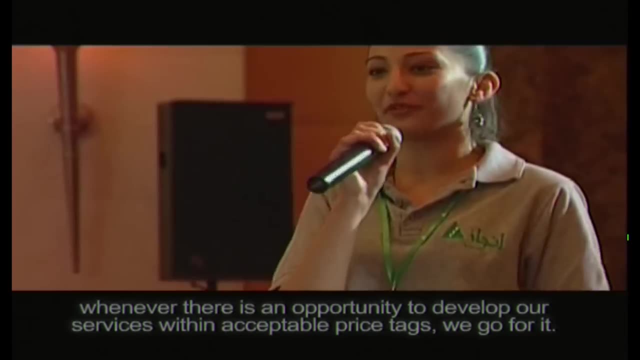 The more we see that there is room for product development, the more we develop it, And the more there is room for us to adjust our prices to match the current market price, the more we do it. We are very flexible in these two areas. 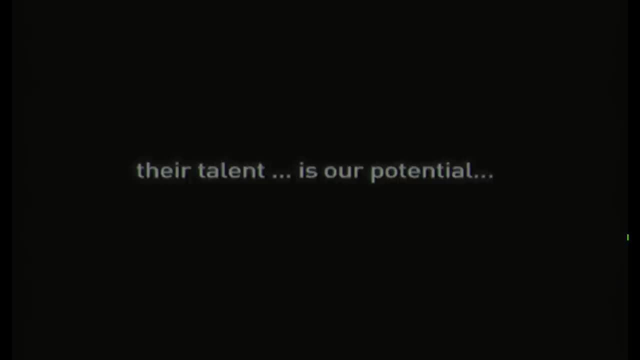 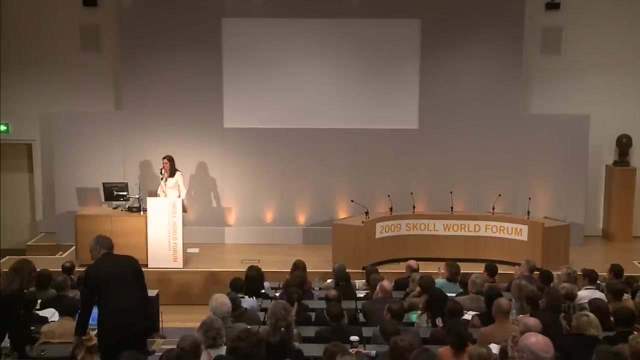 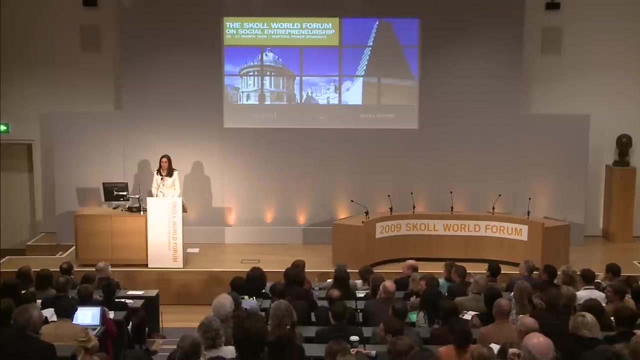 We are very flexible. So I said of course it's a female right. I mean, 50% of the population of the Arab world is female. It's about time they rise. I just wanted to explain a little bit. 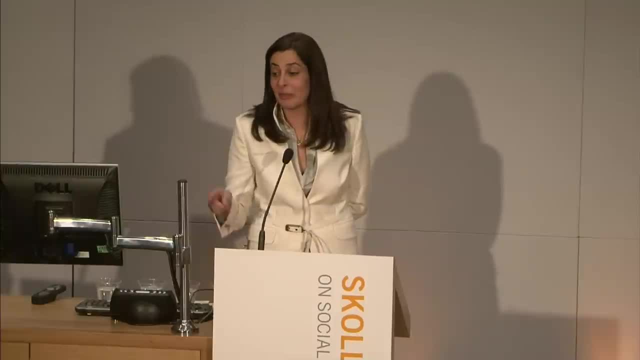 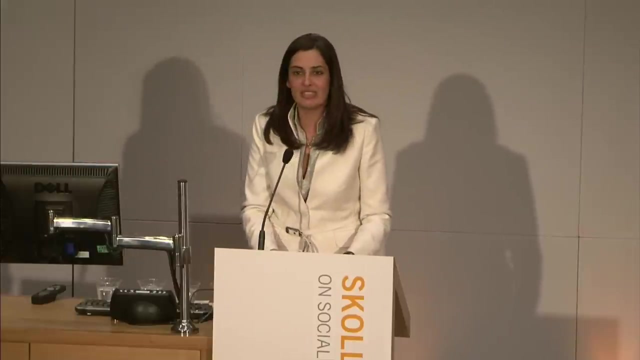 The Arab Bank had taken a public school classroom in Ramallah- 27 girls- and incubated their company right there on their premise. Their HR department of the student company was tied to the HR department of the Arab Bank. Their production department was tied to the operations. 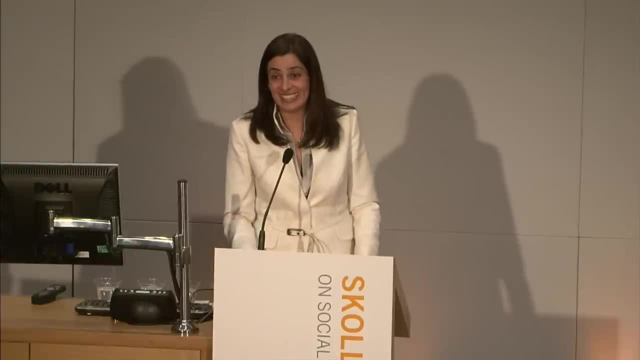 When those judges tested them for three whole days, they knew about stock options and how they're going to go public and their price share earnings And I don't know what. It was such an out of place. It was such an outstanding phenomenon to see them just rise to the top. 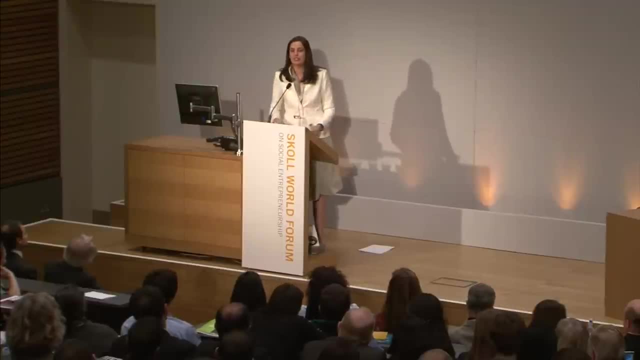 And the females when we welcomed them into Jordan. this was our first regional competition, because in 2007, we finally did have a region of 12 countries, So the first team would come in a girl's team. Where are the boys? 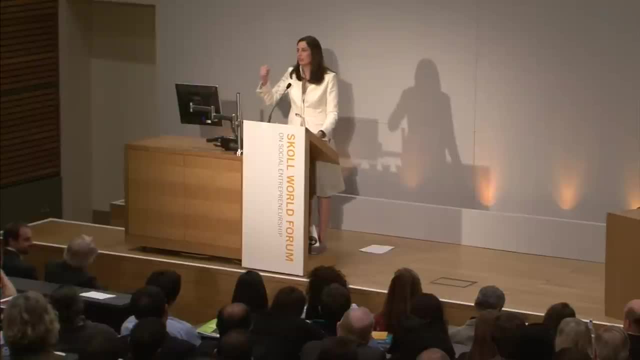 The next country, a girl's team. They really took on to it as their resident debt to prove to their society, to their families, that they can be entrepreneurs and they can be business leaders. When Jeff the other day asked me, I asked him. 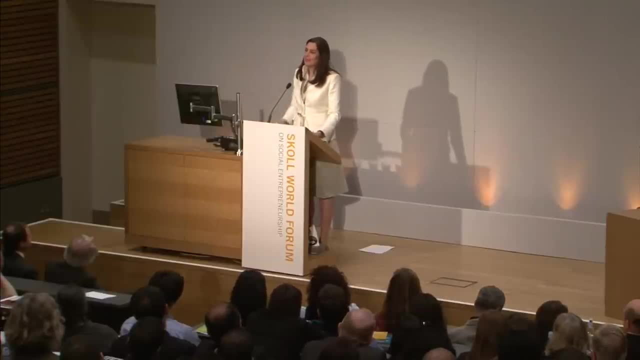 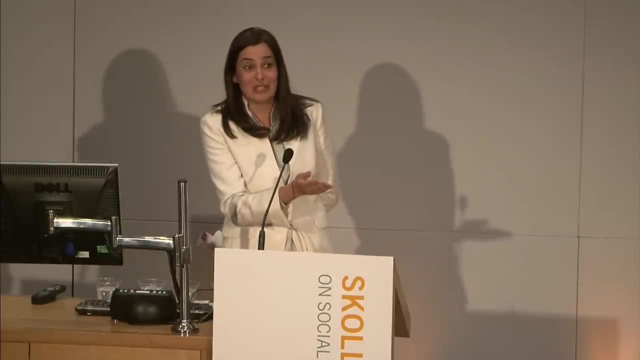 I said what He said. you have a top priority- peace in the Middle East- And I asked him: how was he going to solve it? And he said: that's why we voted you. as a social entrepreneur, I just wanted to fight. 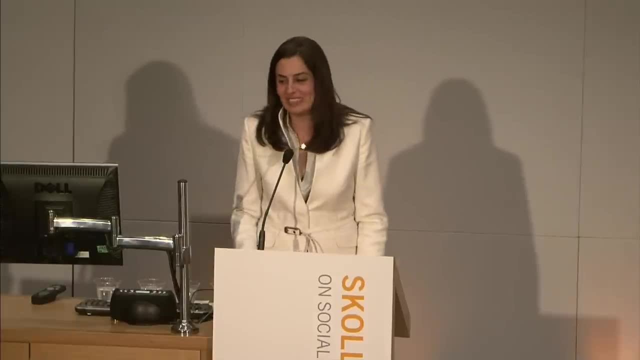 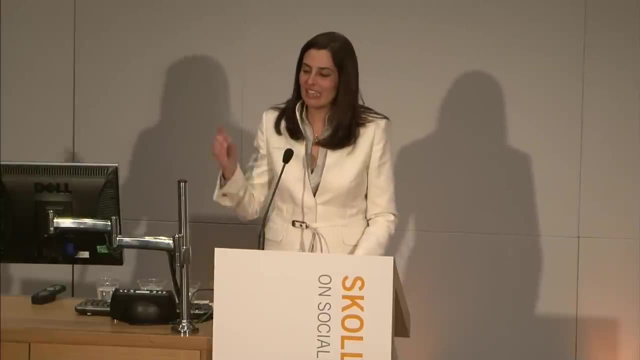 And I tell you, Jeff, that, with one million youth each year, that they are going to be the ones that create peace and prosperity in our region. And with that, I'd like to just read from Khalil Gibran, One of our great philosophers of the Arab world. 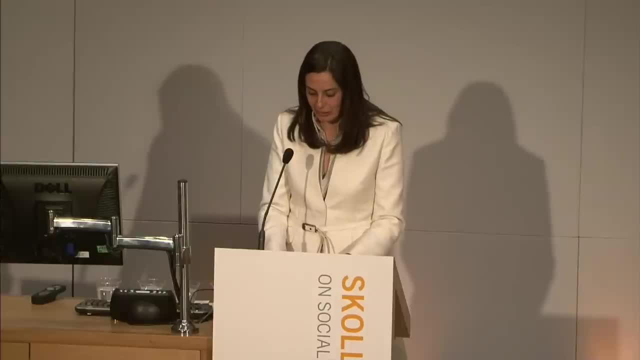 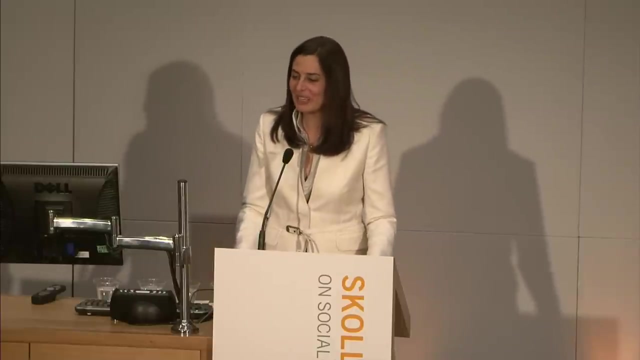 And he says: you work, that you keep pace with the earth and the soul of the earth, For to be idle is to become a stranger onto the seasons and to step out of life's procession that marches in majesty and pride. I want to thank you, Jeff, for giving our youth a chance to march in majesty and pride. 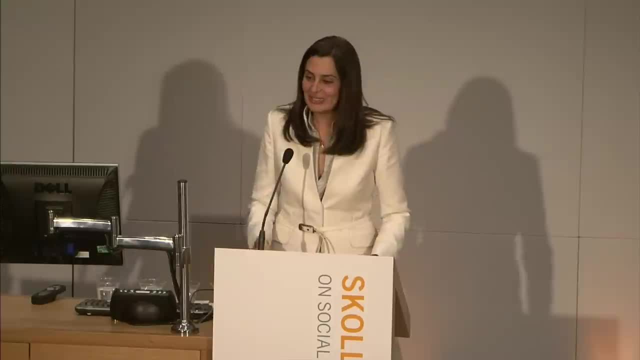 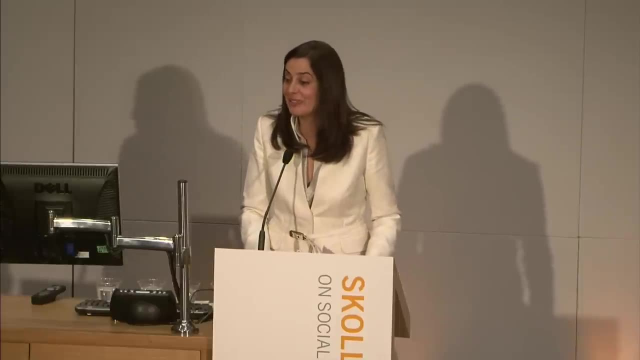 And I would like to invite you to this podium here To give you a book, because from the land of the prophets, you are the modern day prophet that has reached every corner of the Arab world, And this is Khalil Gibran's book. Thank you.